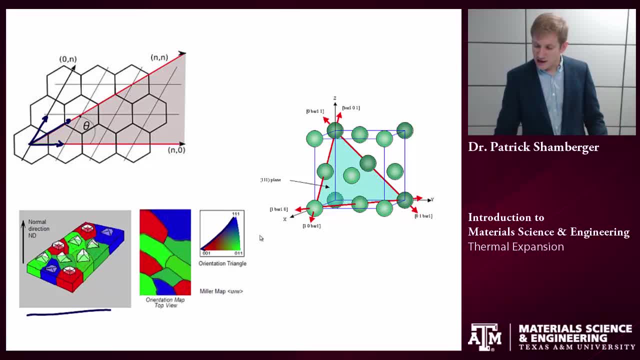 of the grain that's coming out of the plane And I'm giving those a color based on this three-dimensional color scheme here. Finally, something we'll talk about quite a bit later on is close-pack direction. So these are directions along close-packed planes And these are important because slip 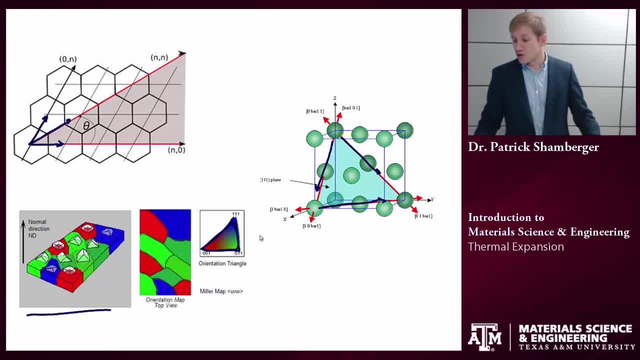 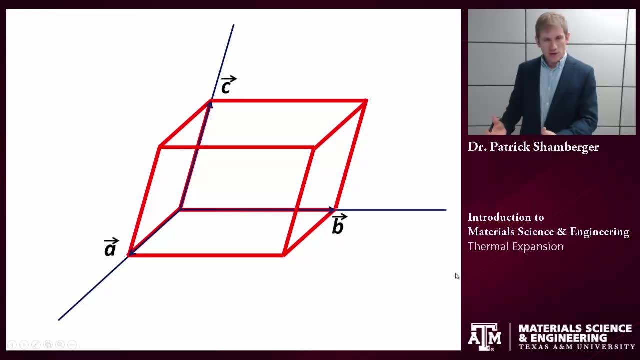 happens along these directions, And so, in order again to talk about these, I need to know how to talk about directions in a crystallolattice. So let's try some examples here. I'm going to start off with a very general lattice. So this is a triclinic lattice. If you can do it in this lattice, you can do it in any. 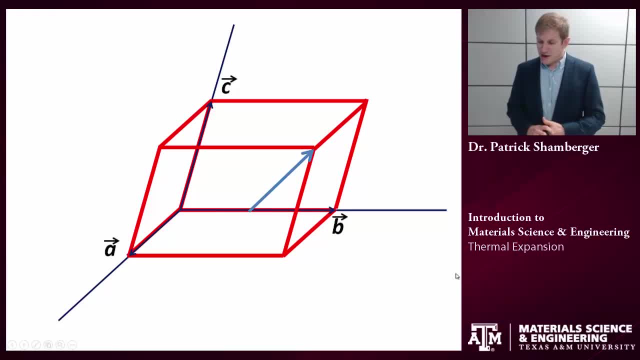 lattice, So I have some direction that I'm interested in. There's different ways to do this, so we're gonna do them both. The first is using the head-to-tail method, And so, basically, I'm describing this vector by subtracting the position of the tail. 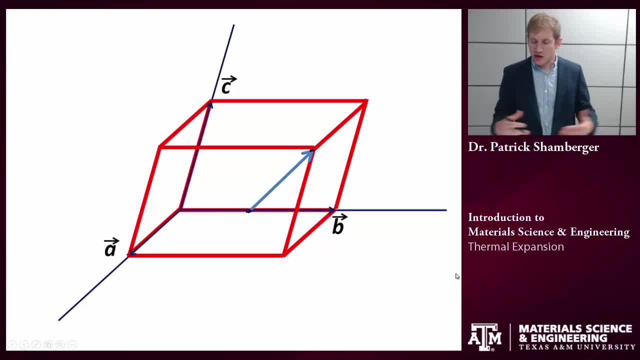 from the position of the head. So again, remember, we talked about how to index points in space. The point of the head here is given by one, one, one, One one. The point of the tail is given by zero, one-half zero. 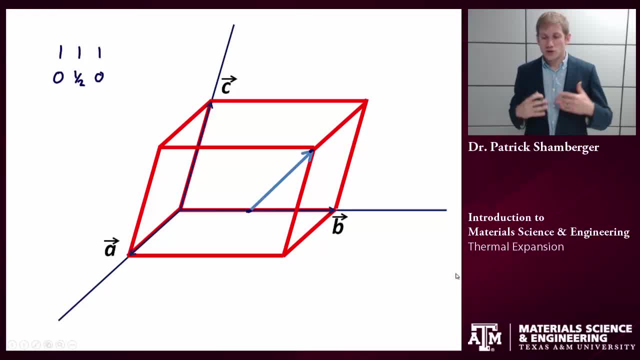 Now, if you don't know how to do this, go back and review the video talking about indexing of points. So if I subtract the tail from the head, I get one one-half one. Now, the final thing I need to do is to write this in the typical vector direction notation. 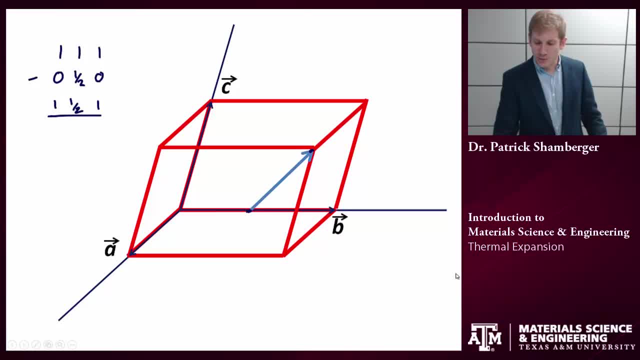 And so what I wanna do is I'm gonna remove any fractions, So I'll multiply through by two. That gives me two, one, two, And because this is a direction, I'm using square brackets to denote this. Okay, so another way to do this same direction. 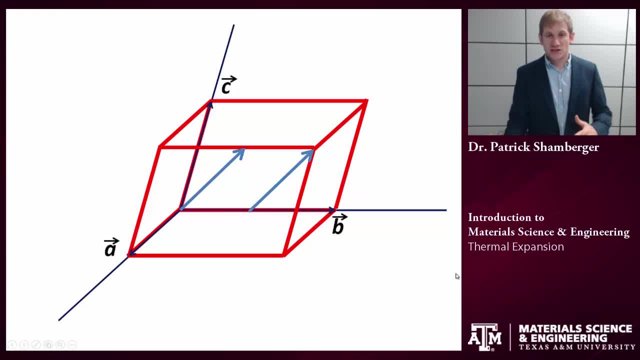 Again, I can shift a direction. The absolute position is not important, just again the direction. So these two are equivalent. But if I take any direction and I shift it such that the tail is sitting on the origin, then if I'm using the head minus tail method, 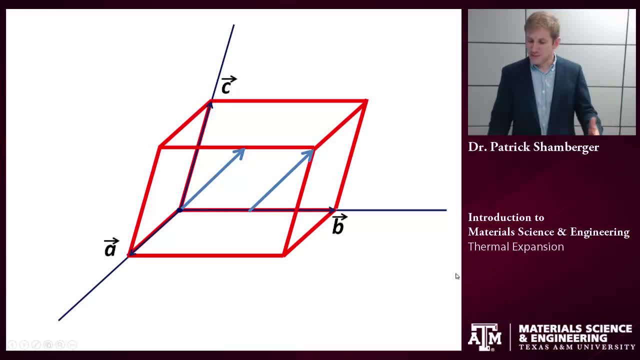 I'm subtracting zero, zero, zero from the head position, So this is sometimes a little bit easier. So I shift the direction so that the tail sits on the origin, and then all I need to do is figure out the fractional coordinates of this head position. 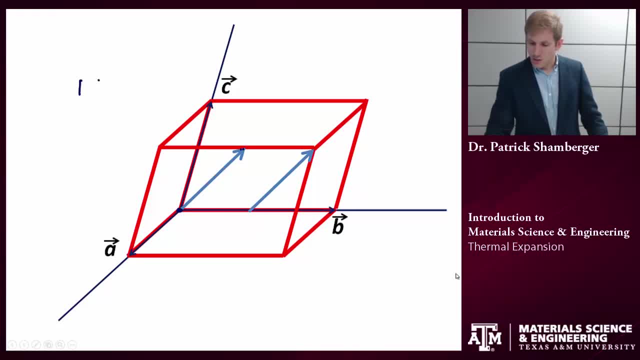 And so in this case it's one, one-half one. Again, if I want to write a direction, I want to use integers, not fractions, and I need to use the square bracket notation. So I multiply this whole thing through by two. 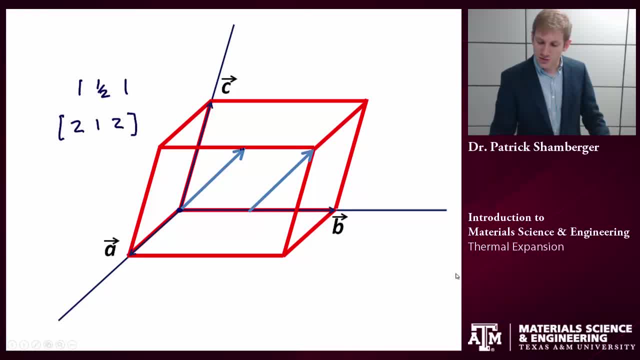 and get two, one, two, and I use square brackets, And this is how I would denote this particular direction that I'm showing And notice that this is the same thing we got using the previous method. Okay, now what about if you're given a direction? 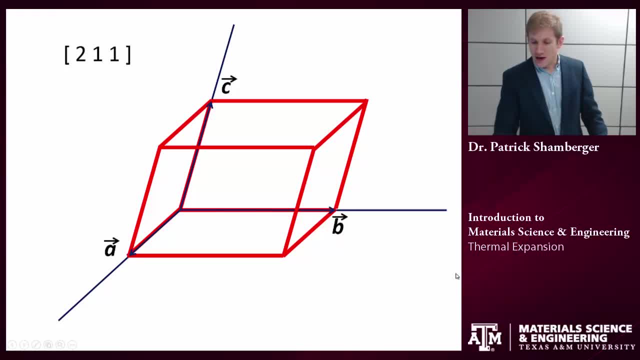 and you're asked to draw that on a unit cell. So again, there are two different ways to do this. We're going to do these sequentially. First is if I want to keep this direction entirely within the one unit cell, And so this is essentially the exact opposite. 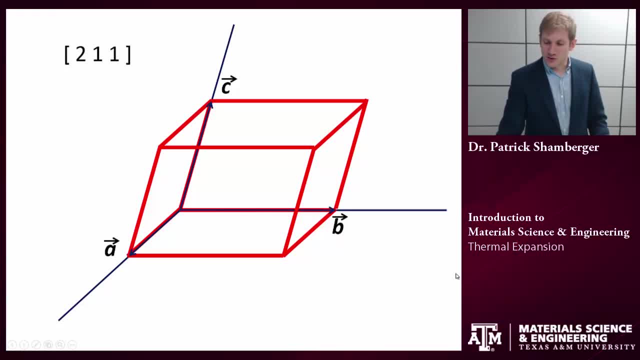 of the process that we just did. So I need to divide through so that all of these numbers are less than one. So if I divide this whole thing by two, I get one, one-half, one-half, And this is going to be the position of the head. 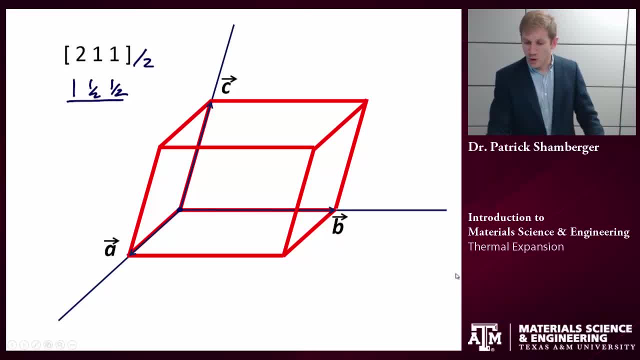 of that direction. So I can start at the origin and I can start at the head. I can start at the origin and I can go to one, one-half, one-half. So one is the fractional coordinate in the x direction. 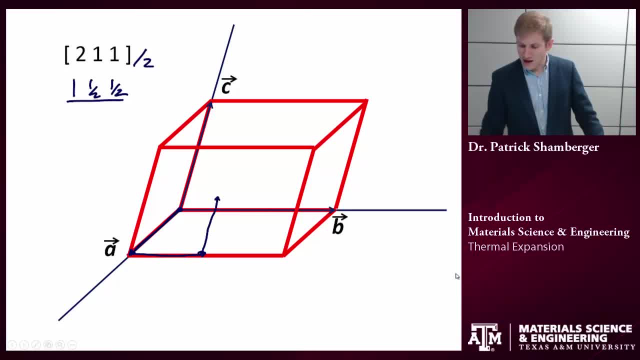 one-half in the b direction and one-half in the c direction, And so this is a vector. It goes from the origin to the exact middle of this front face. Okay, let's try the other method In this case. I'm not going to reduce it. 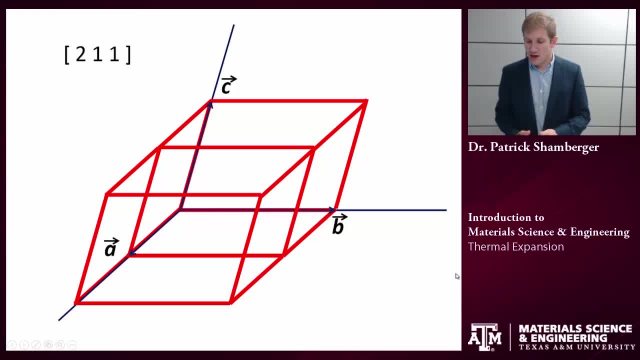 so it's sitting entirely within one unit cell I'm going to use. I'm basically going to extend and use the unit cell neighboring it forwards out of the plane here And I can do the same exact thing. So, again, this is going to give us. 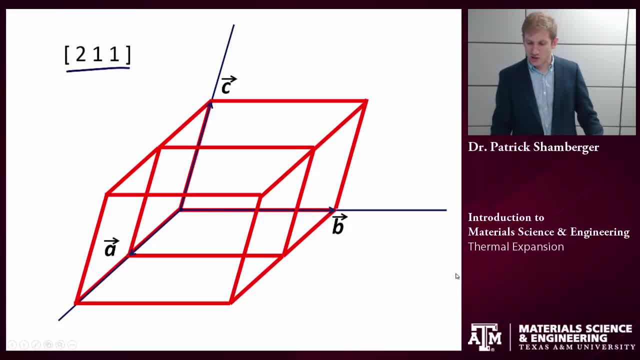 the position of the head of the vector and the tail is going to sit on the origin. So two is all the way down here, One is all the way up here And one is all the way up here, And so this is a vector that goes from the origin all the way.